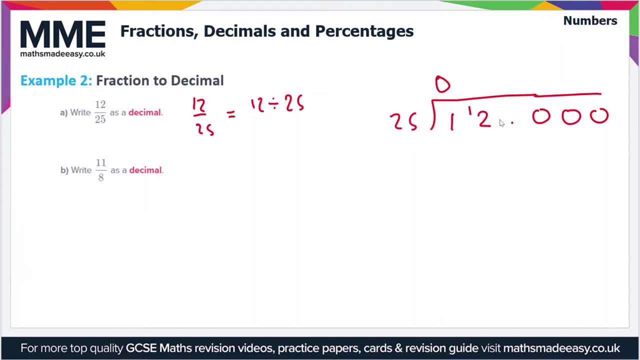 the 1 forward. And then again we've got: how many times does 25 go into 12? this time And again, the answer is zero. So we put a zero here and carry the 12.. Let's put our decimal point in. So now we have: how many times does 25 go into 120?? The answer is 4.. And then 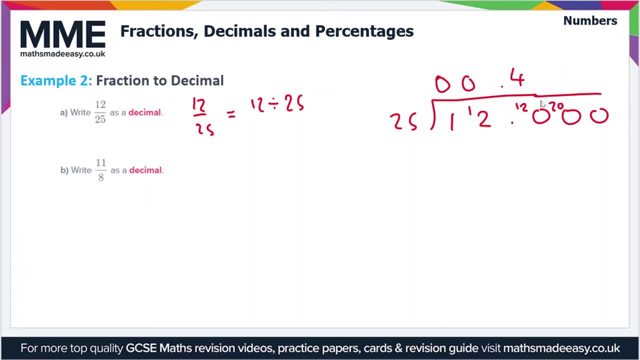 we're left with 20 as a remainder. So 4 times 25 is 100. So 120 minus 100 is 20.. So that's why we have a remainder of 20.. And then finally we have: how many times does 25 go into 200?? 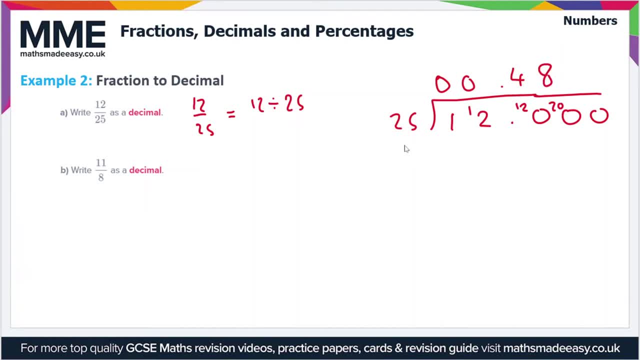 And the answer is 8.. And there's no remainder, So our answer is 0.48.. So moving on to part B, then, And we have to write 11 over 8 as a decimal, So 11 over 8 is equal to 11 divided by 8.. So, again, we're going to use the bus. 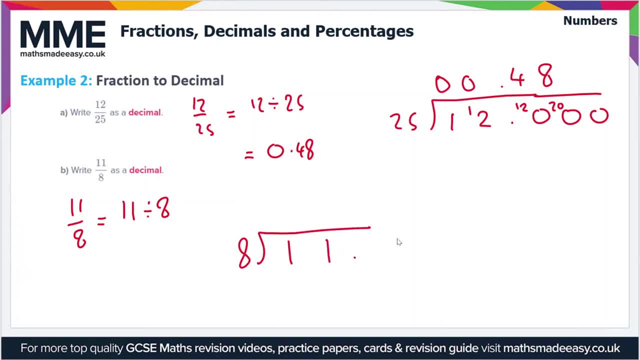 stop method here. So we've got 8 into 11.. Let's put some zeros in. So first of all, how many times does 8 go into 1?? The answer is zero, So we'll carry the 1.. Then we have. 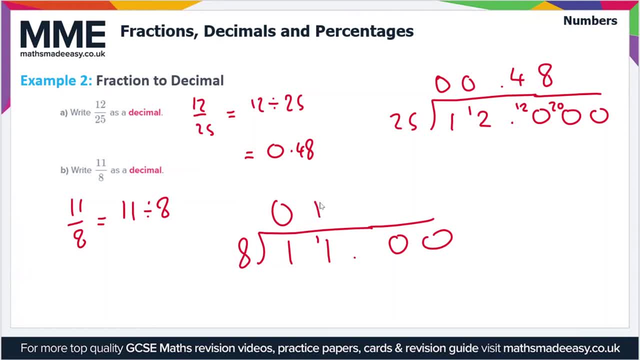 11 here. So how many times does 8 go into 11?? The answer is once, And we get a remainder of 3.. So how many times does 8 go into 30? this time The answer is 3 times, So I'll put my decimal point back in: So 3 times. 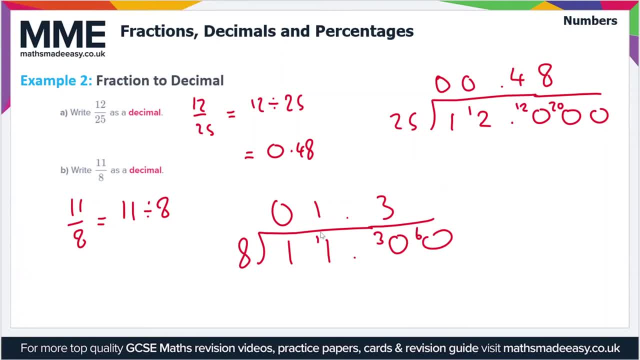 8 is 24.. That gives us a remainder of 6.. So how many times does 8 go into 60? now The answer is 7.. So 7 times 8 is 56.. So we put 7 here. So 60 minus 56 is 4.. So we have a. 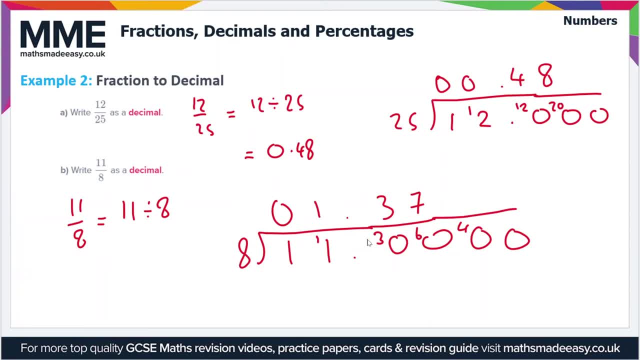 remainder of 4.. Let's put some more zeros in, So now we have: how many times does 8 go into 40?? The answer is 5.. We don't have any remainder here, So 11 divided by 8 is equal. 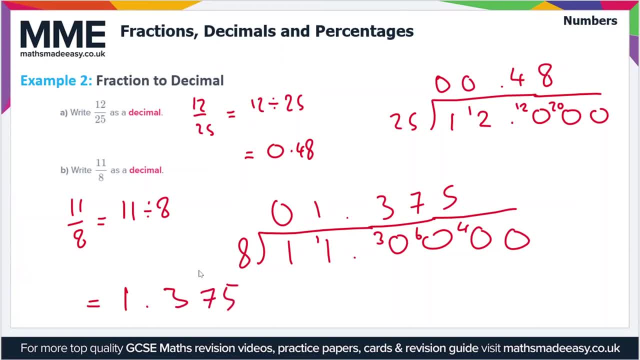 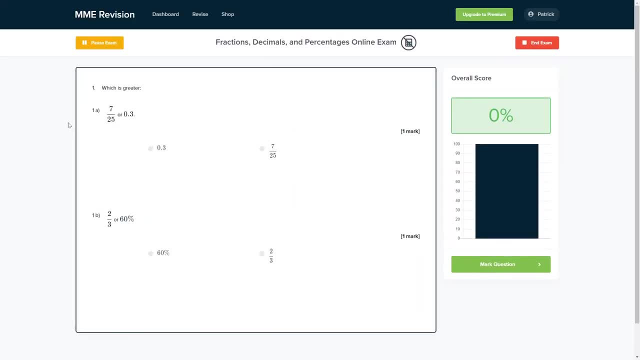 to 1.375.. If you're feeling good on this topic and you want to get some practice in, you can do so with our online exam. It's available through our revision platform. So here you'll find loads of different questions to have a go at. So there's a variety of different. 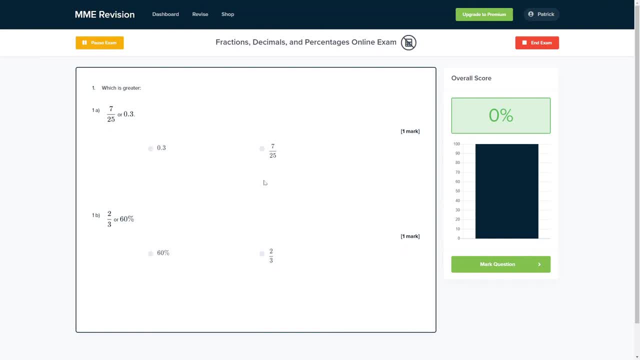 question types as well, and you'll get instant feedback on each and every one of them. So it's a really good way of keeping track of where your weaknesses are and where you can find them. So if you're confident and ready to take the test, then click the link below.